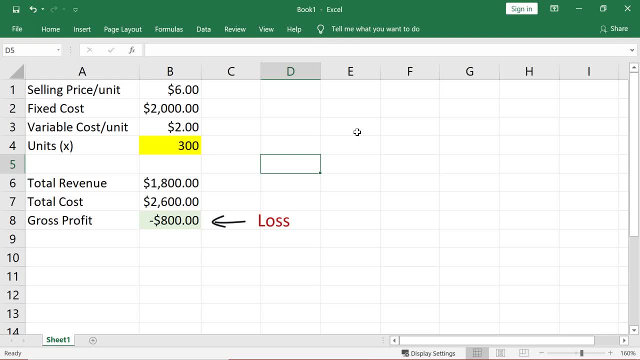 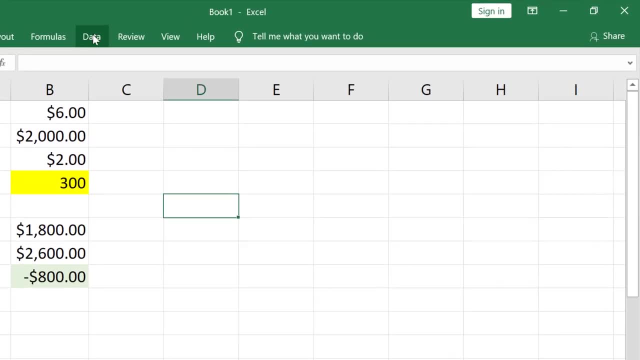 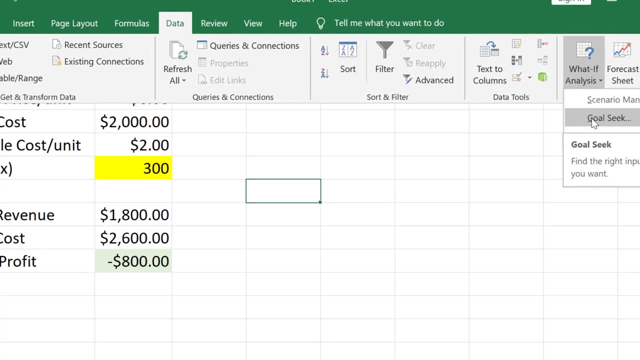 As you can see here, we have a loss of $800.. Now let us determine the number of units required to break even using Goal Seek. Click on the Data tab. What If? Analysis, then Goal Seek? Since our objective is to determine the number of units, that will be a change in. 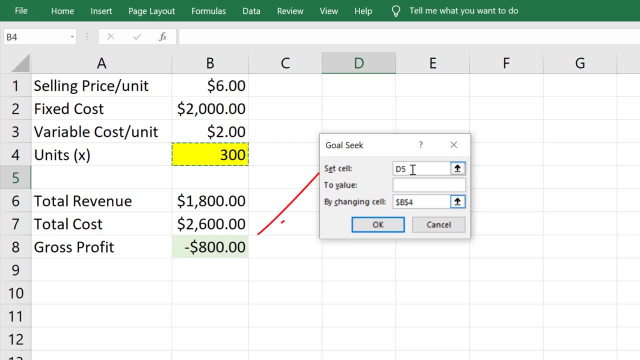 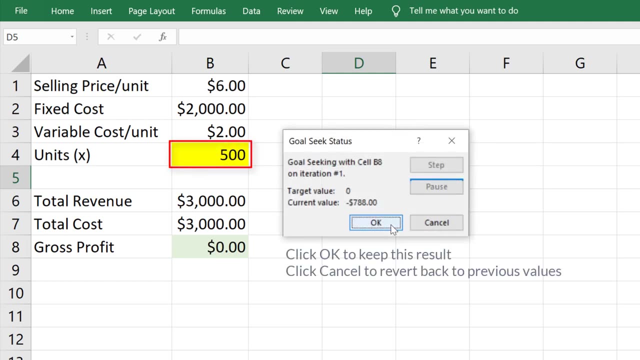 cell To break even we have to set profit to zero. So our set cell is the one containing profit and to value 0. Click OK. And we have 500 units at break even point. I'm going to click OK. Now suppose I want to find the selling price required to make a profit of, say, 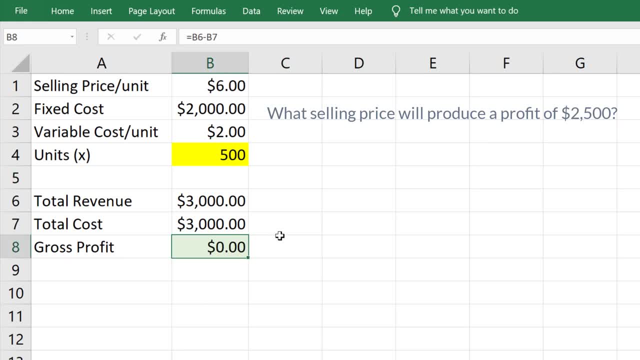 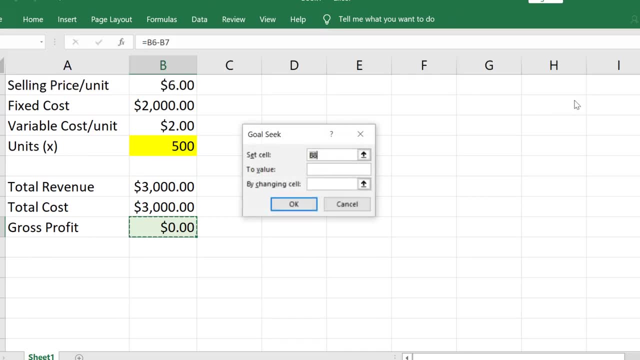 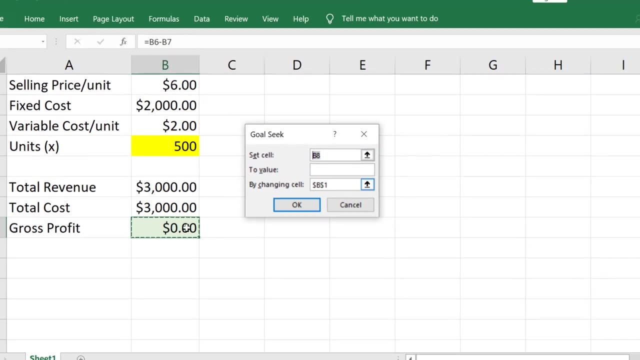 $2,500.. unit at 500.. Then I'll go to Data. What If Analysis? then Goal Seek. again. This time I want to determine the selling price. So my changing cell will be Selling Price And I will set the profit cell to 2500. 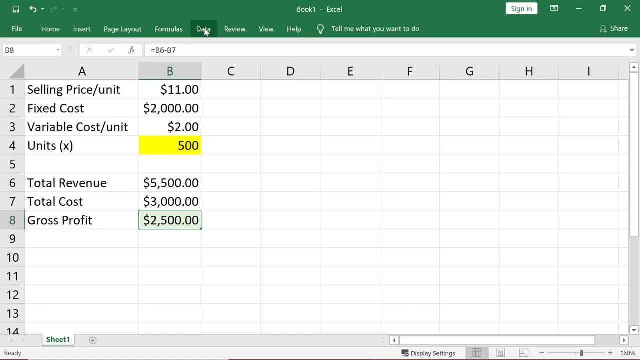 And clicking OK gives a selling price of $11.. In conclusion, to use Goal Seek, the said cell must contain a formula that is linked to the changing cell. The changing cell, however, must be an input value and not a formula, And that's it. Thanks for watching.